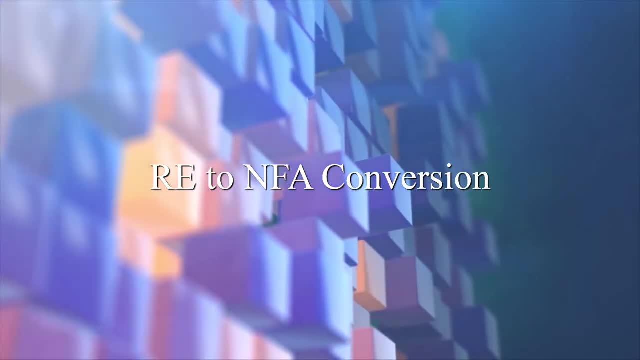 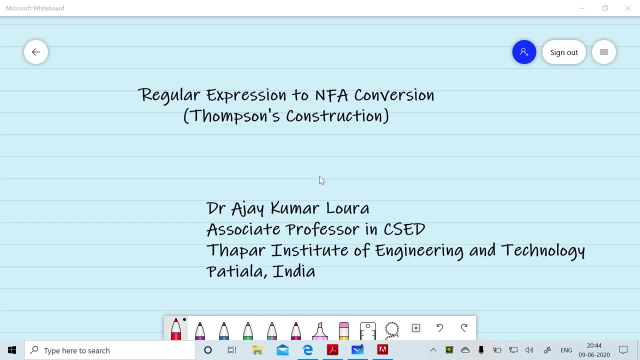 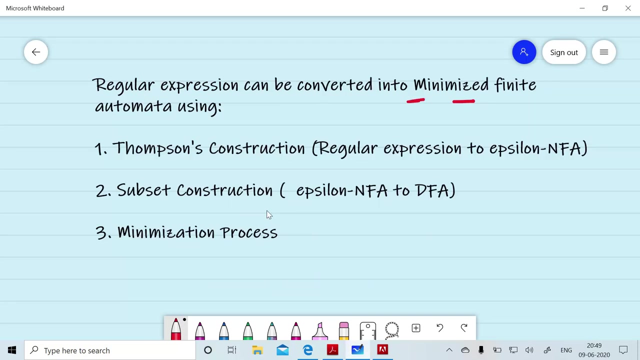 Welcome to the session. Regular Expression to NFA Conversion. I am Ajay Loora. In this session we will discuss the assumption construction for the conversion of regular expression to epsilon NFA. A regular expression, R, can be converted into minimize finite automata using following three steps. In the first step, we will apply: 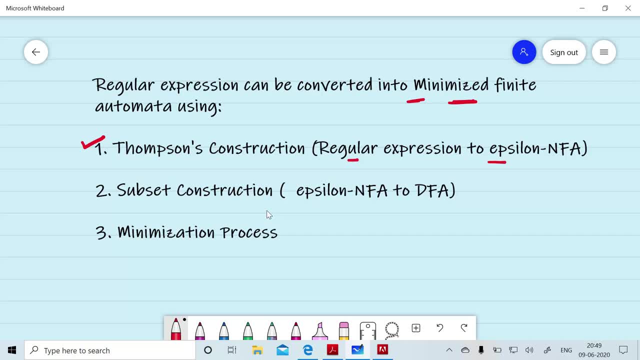 assumption construction to convert a regular expression into epsilon NFA. In the second step, we will apply subset construction to convert epsilon NFA into DFA And in the third step we will minimize the DFA. In this session we will discuss the first step to convert. 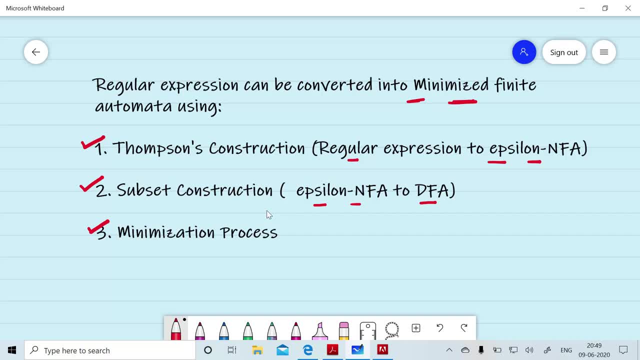 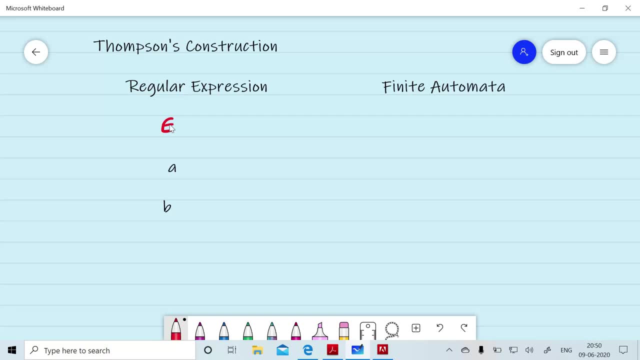 regular expression into epsilon NFA using assumption construction. Suppose we have a given regular expression, NULL. It can be represented by a finite automata with two states. One is the initial state and on reading of NULL we will move to the final state. If our given regular expression is symbol A, it can be represented by two. 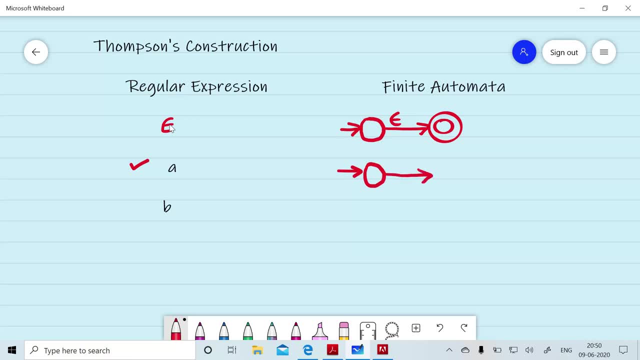 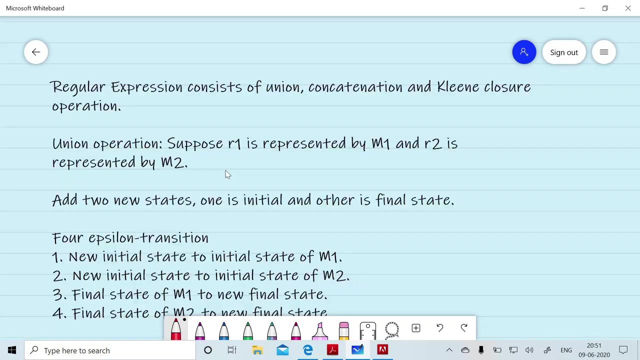 states. One is the initial state and on reading of symbol A, we will move to the final state. Similarly, if we have a regular expression B, then it can be represented by two states: starting state and on reading of B, we will move to the final state. A regular expression. 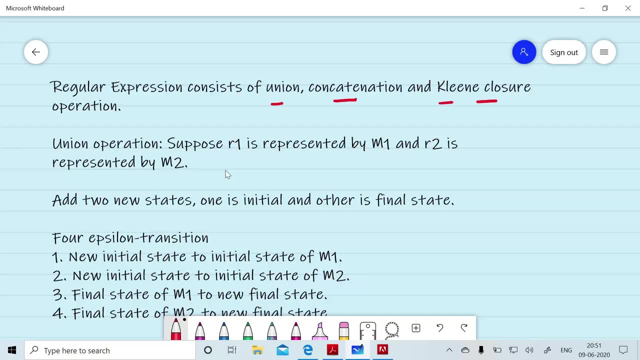 consists of union concatenation and clean closure operations. Now we will discuss the union operation in case of assumption construction. Given a regular expression R1,, suppose it is represented by finite automata And regular expression R2, that is represented by finite automata M2.. For performing R1 plus. 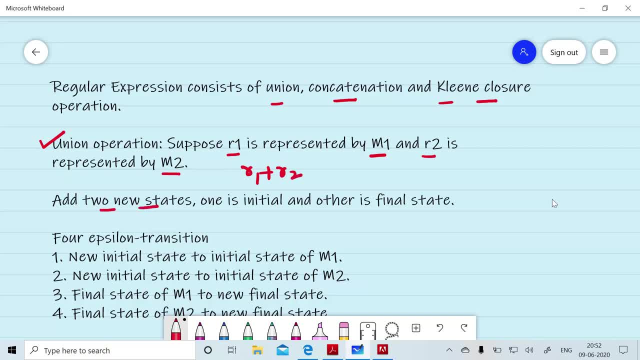 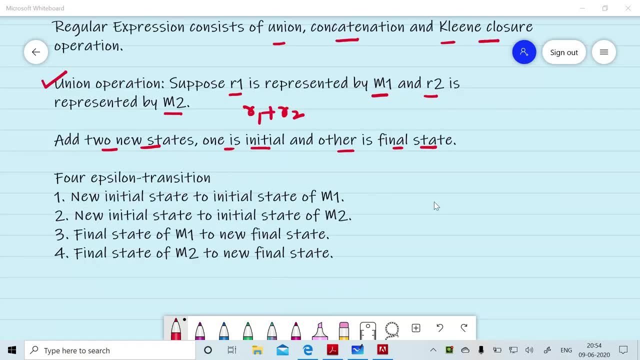 R2, we need to add two new states. One is known as initial state and the other is known as the final state. So we need to add four epsilon transitions. First one is from the new initial state to the initial state of M1.. Suppose this is the finite automata for 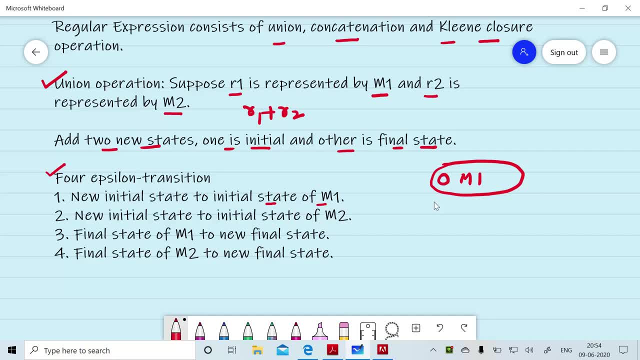 M1.. With the initial state as this one and final state as this one, And this is the finite automata for M2.. With the initial state as this one and this is the final state. So we will add two new states, One as the starting state, another as the final state. We will 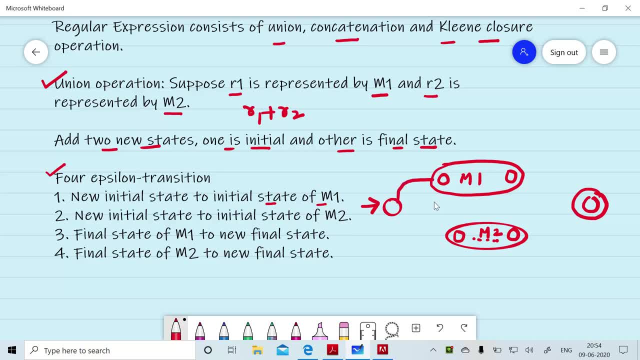 add four new transition: from this new initial state to the initial state of M1.. From this new initial state to the initial state of M2.. M2- from final state of M1 to the new final state. from final state of M2 to the new final. 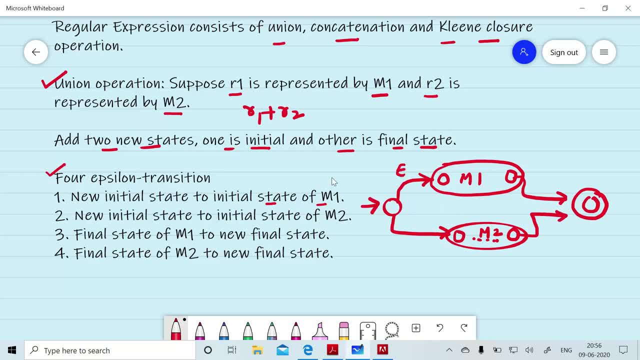 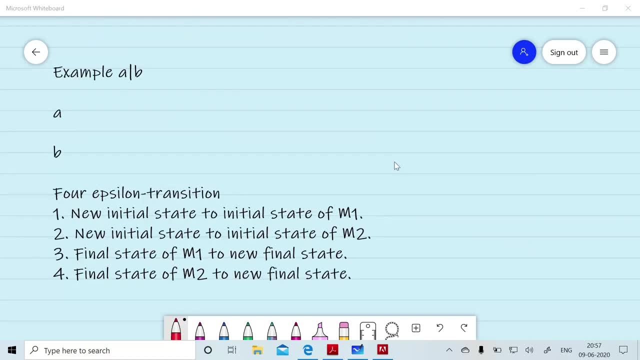 state. all these four transition are null transition. suppose we want to convert A or B into NFA using Thomson construction. so A can be represented by two state, one is the initial state and another is the final state. B can be represented by two states, one is the initial state and. 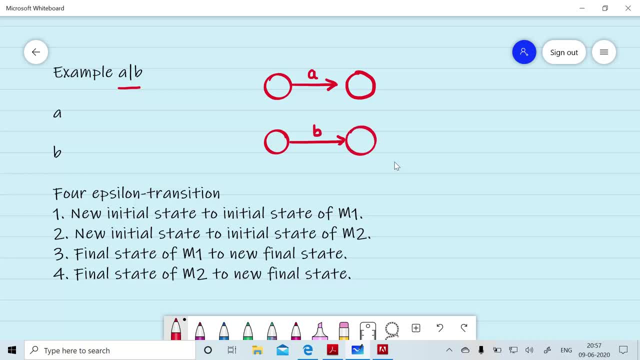 another is the final state for performing union operation. we will add two new state: one is the initial state and the another will be the final state. we will add four: transition: from new initial state to the initial state of A, from this new initial state to the initial state of B. from final state of A to the new final state. 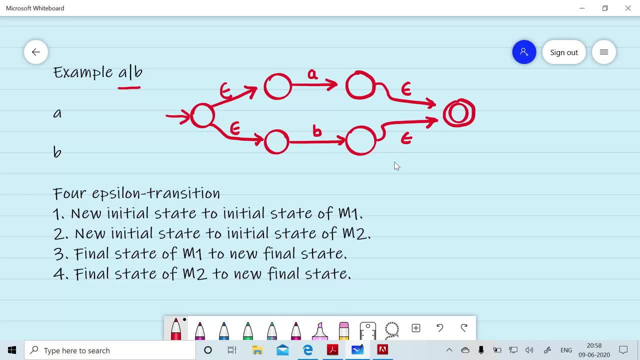 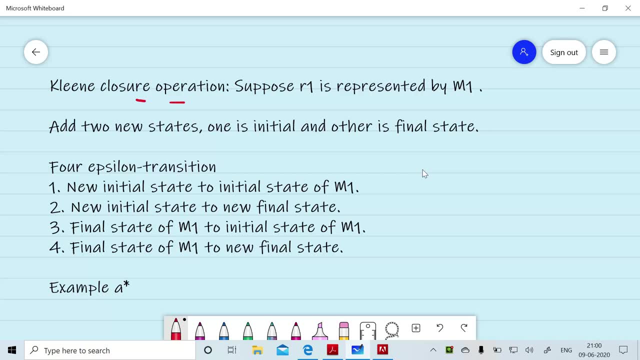 from final state of B to the new final state. now we will discuss how we can able to carry out clean closure operation using Thomson construction. suppose a regular expression R1 is represented by finite automata M1 using Thomson construction. for performing R1 star we need to add two new state. one is the initial state and the another will be the final state. 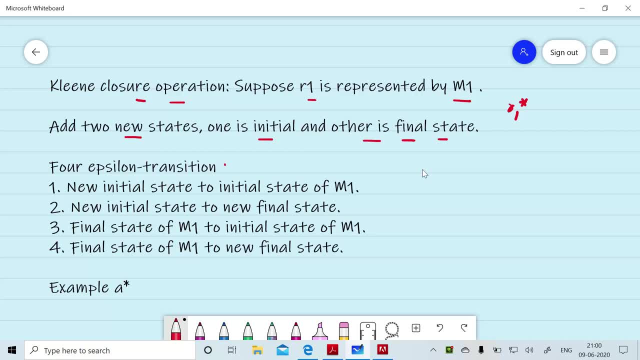 we will add four epsilon transition. for example, for A star, A is represented by two states: one is the initial state, another is the final state. we need two new states: one is the initial state and another is the final state for performing and another will be the final state for performing a star. we will add two new. 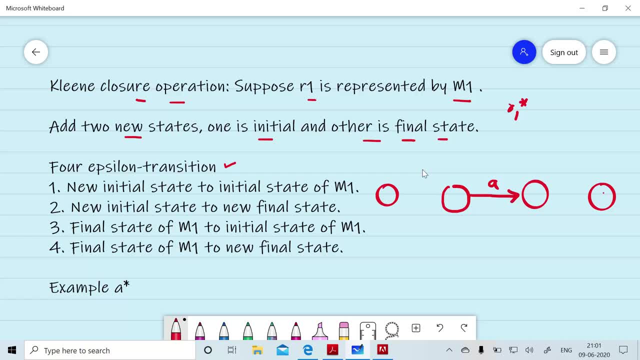 state. one is the initial state and another will be the final state. we will add four transition. first one is from new initial state to the initial state of m1. we will add a null transition. in the second one- new initial state to the new final state- we will add this transition. third one is from the final. 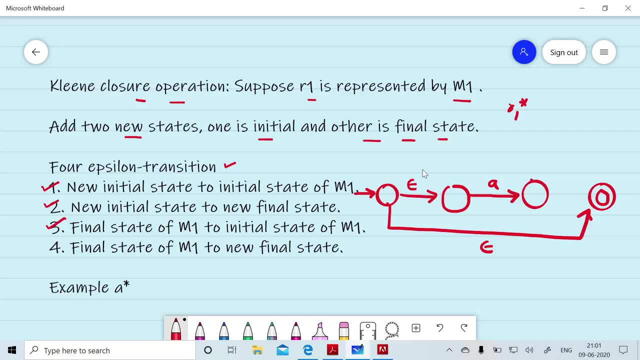 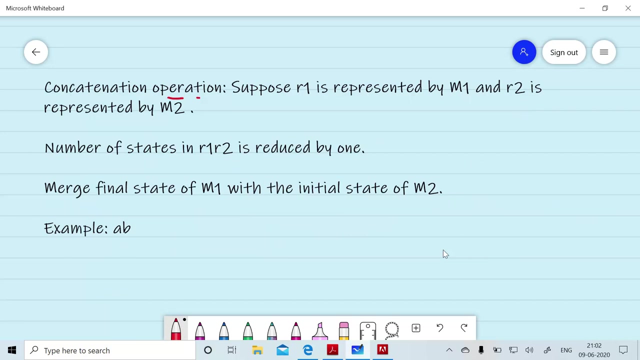 state of m1, that is, this particular state to the initial state of m1. fourth, one is from final state of m1 to the new final state and it represent a NFA for a star. now we will discuss how we can able to carry out concatenation operation using Thomson construction. 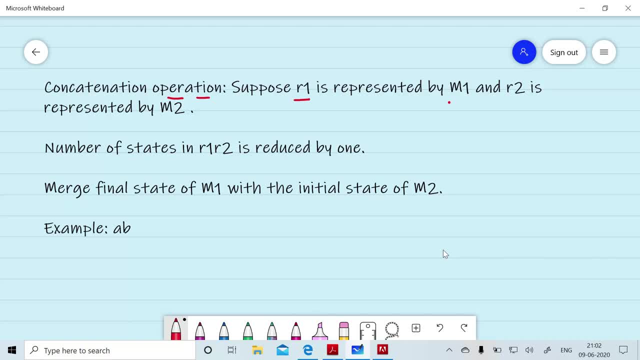 given a regular expression R1 and its equivalent NFA m1 using Thomson construction and regular expression R2 and its equivalent NFA m2 using Thomson construction, we are interested to apply R1- R2, that is, concatenation of R1 with R2, so in concatenation operation number of state is reduced by 1 in. 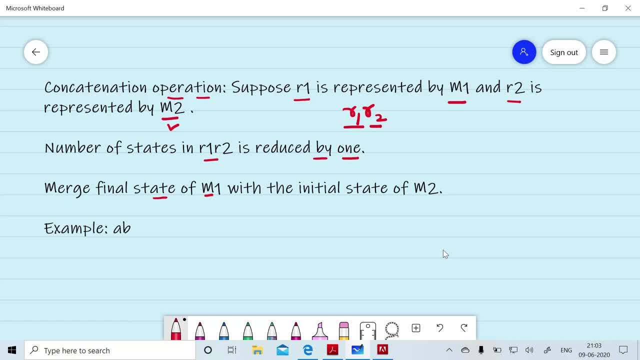 concatenation operation, we will merge the final state of M1 with the initial state of M2.. For example, for regular expression, AB. A can be represented by two states. One is the initial state, another will be the final state. B can be represented by two states. 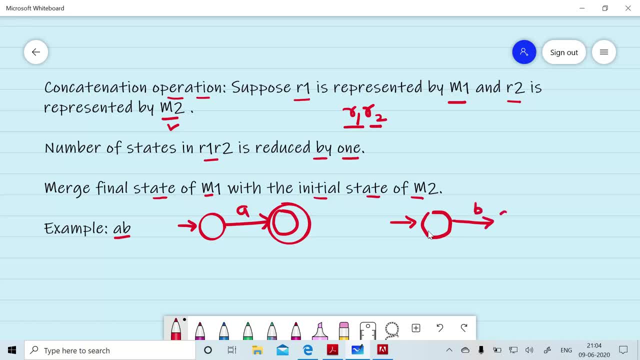 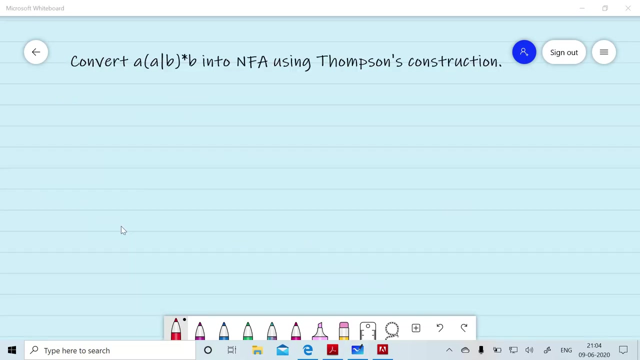 One is the initial state, another will be the final state. Now AB can be represented by: we will merge final state of A with the initial state of B, So total number of states will be reduced by one in case of concatenation operation. Now we want to convert the regular expression A into A plus B. 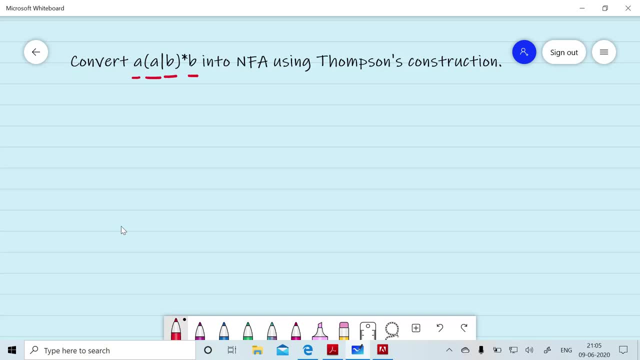 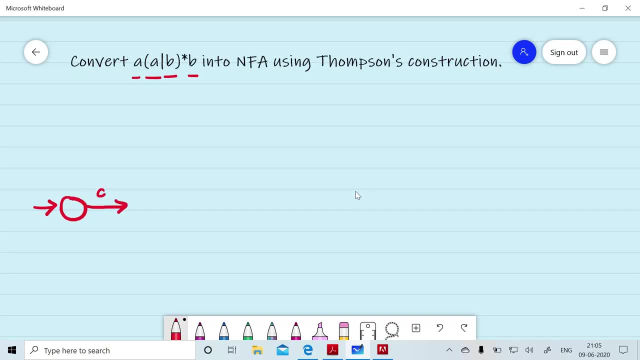 Now, first we will design A into A plus B, C, Then we will carry out the union operation A or B. So we will add two states. One is the initial state, another one will be the final state. We will add four null transitions. 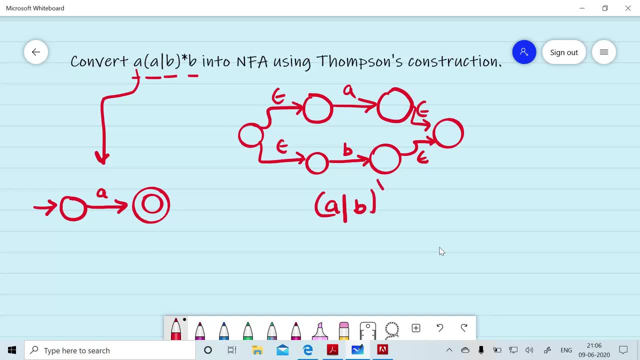 Now we want to perform A or B star, So we will add two new states. This one will be the initial state, this one will be the final state. We will add a null transition from new initial state to initial state of A or B. 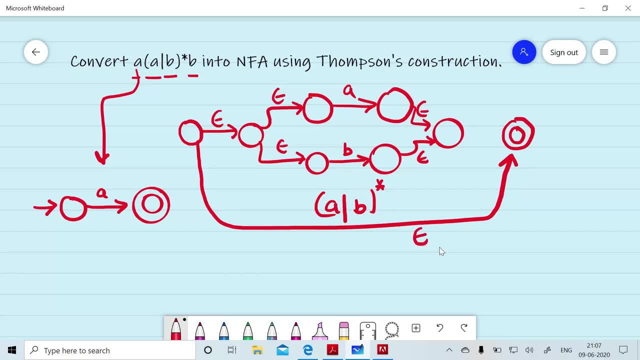 We will add null transition from initial state to final state. We will add a null transition from final state of A or B to initial state. We will add a null transition from final state of A or B to initial state or B to the new final state. Now we need to concatenate A with A or B star, So we will 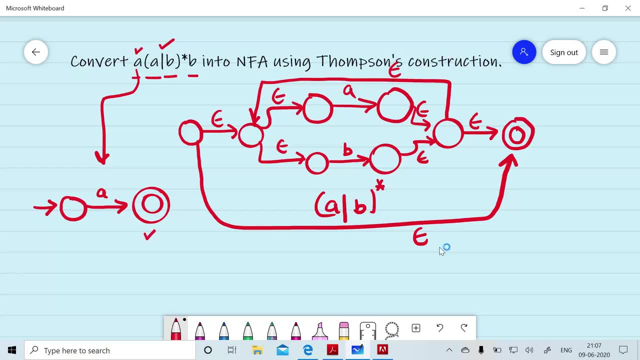 combine the final state of A with the initial state of A or B star, because in the concatenation we will merge the final state of R1 with the initial state of R2. So we will merge this state- let's call it as 1- with the state number 2.. So on merging we will get- now we will- 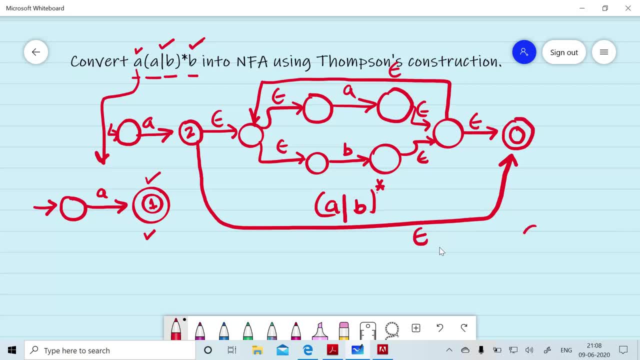 design an FF for B using Thomson construction with two states. One is the initial state and another one will be the final state. Now we have to perform the concatenation of A or A or B star with B, So we need to merge this final state with the initial state of this one. Now this state: 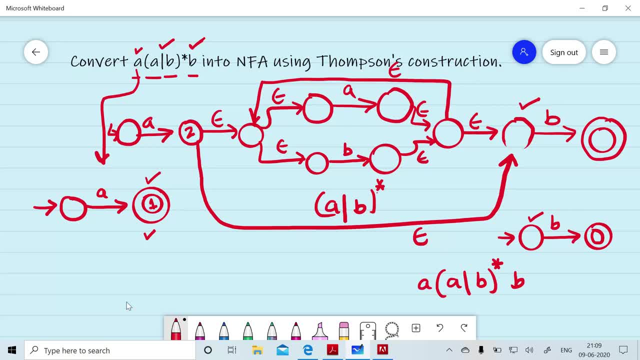 will no longer to be the final state, So this state will become the non-final state. now We can give any names to this state, like 1, 2,, 3,, 4,, 5,, 6,, 7,, 8,, 9,, 10,, 11,, 12,, 13,, 14,. 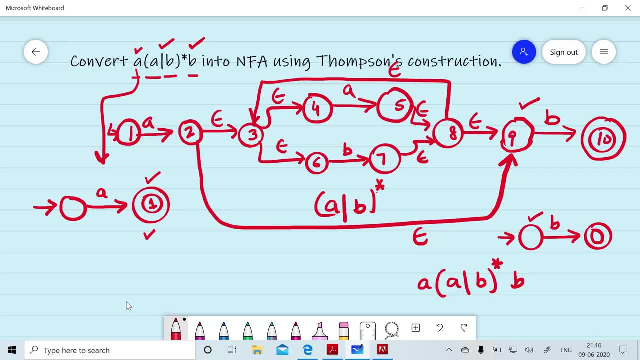 15,, 16,, 17,, 18,, 19,, 20,, 21,, 22,, 23,, 24,, 25,, 26,, 27,, 28,, 29,, 30. And this represents the 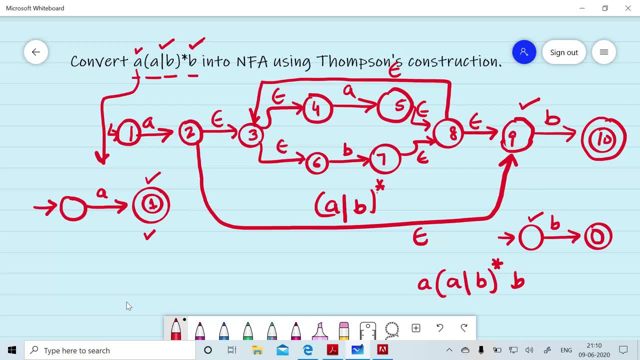 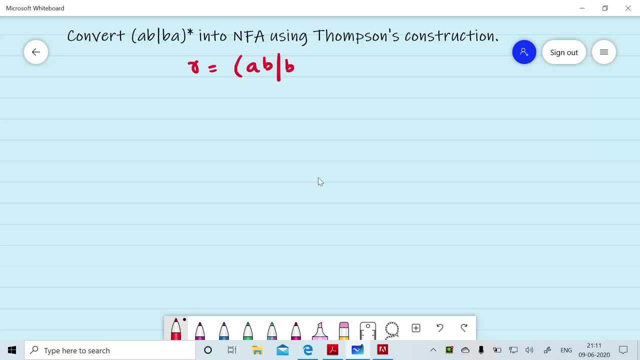 NFA for the given regular expression using Thomson construction. Now, given the regular expression R, AB or BA star, we want to convert this regular expression R, into NFA using Thomson construction. So first we will convert A into NFA. A can be represented by two states. One is the initial state, another one will be the 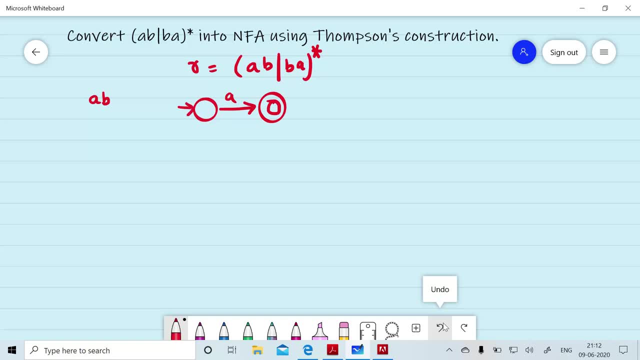 final state. Similarly for B, we need to create two states. One is the initial state, another one will be the final state. Now for AB, we will merge the final state of A with the initial state of B, So we'll get the NFA for us. 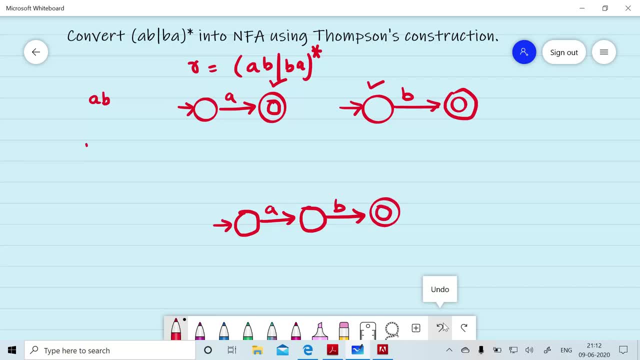 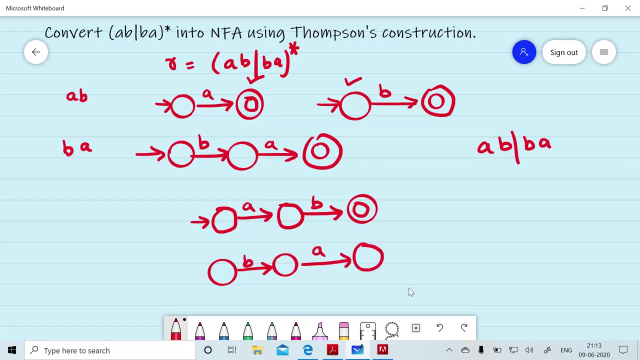 Similarly for BA. we will get this NFA. Now we want to perform union between them because AB or BA. now AB or BA can be represented by. we will add two state: one will be the initial state and another will be the final. 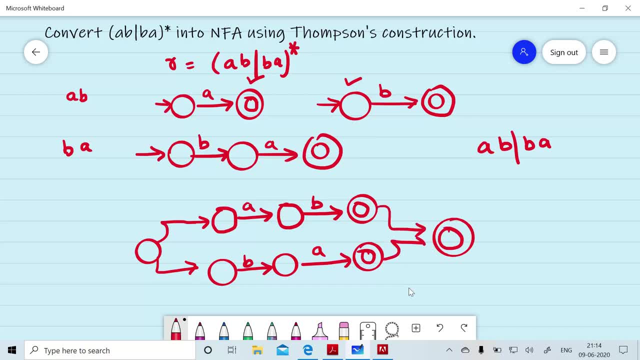 state with null transitions. So this represent a NFA for AB or BA, And now these two state are no longer final states. Now we have to perform plain closure on AB or BA, So we will add two new state. one is the initial state and another one will be the final state.